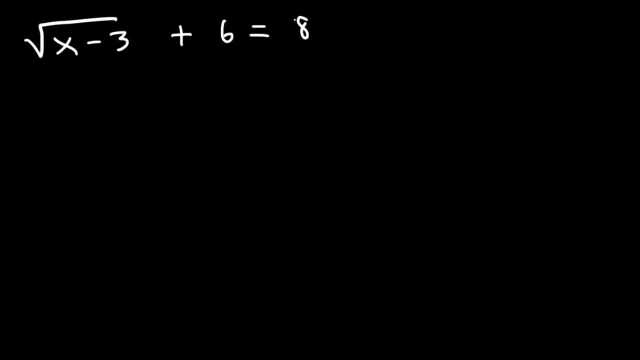 So what can we do in order to solve the variable x? Feel free to pause the video and work on the example. Well, the first thing we should do is subtract both sides by 6.. These two will cancel, and 8 minus 6 is equal to 2.. 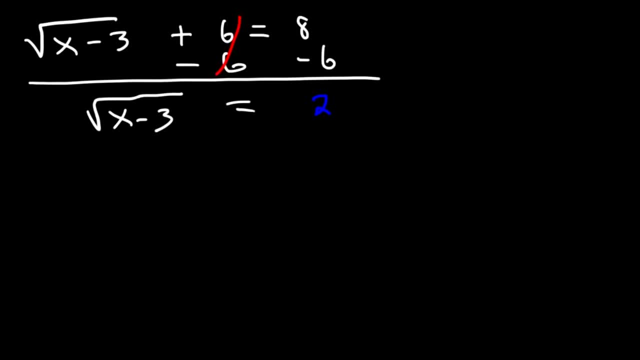 Now, what do you think we need to do at this point? How can we get rid of the square root? In order to get rid of the square root, we need to take the square of both sides. The square. The square of the square root will cancel. The index number is a 2, so these two will cancel. 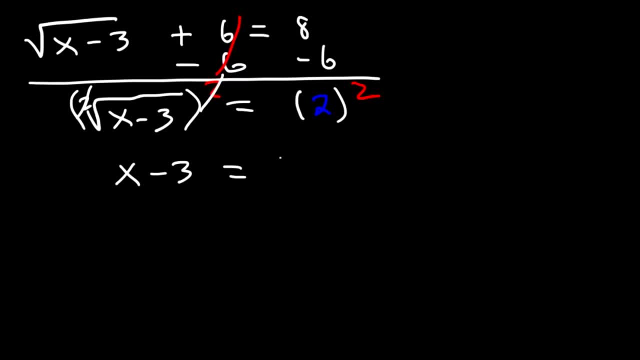 And so you're going to get: x minus 3 is equal to 2 squared, which is 4.. And now we can add 3 to both sides. 4 plus 3 is 7, so x is equal to 7.. This is the answer. 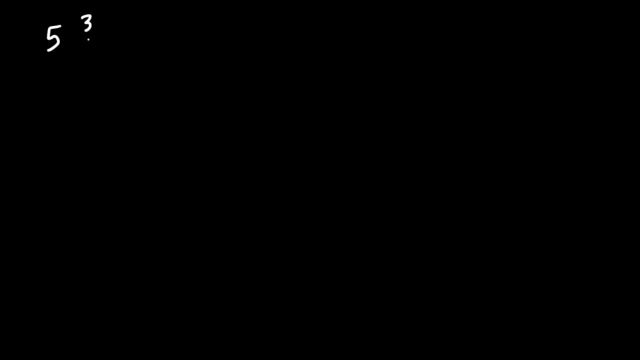 Let's try this one: 5 multiplied by the cube root of x plus 2.. Minus 4 is equal to 6.. For each of these problems, take a minute, pause the video and work on it. Try to solve it yourself first, and then see if you have the right answer. 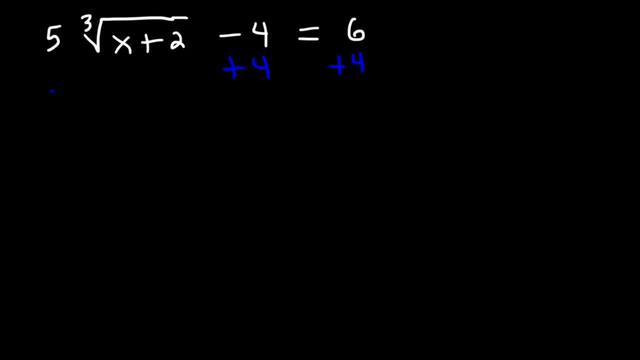 Now let's add 4 to both sides. 6 plus 4 is 10.. So 5 times the cube root of x plus 2, this is equal to 10.. So now, what do you think we need to do at this point? 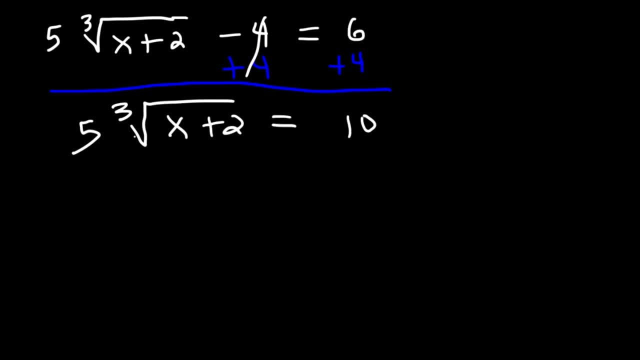 In order to separate The 5 and the cube root expression, since they're multiplied, we need to do the opposite of multiplication, which is division. 10 divided by 5 is equal to 2.. And so now we have this expression. 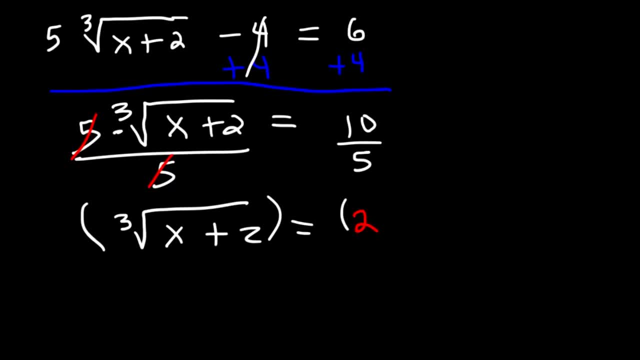 And in order to get rid of the cube root we need to raise both sides to the third power. So on the left we have x plus 2.. Now 2 to the third power is basically 2 times 2 times 2, 3 times, which is 8.. 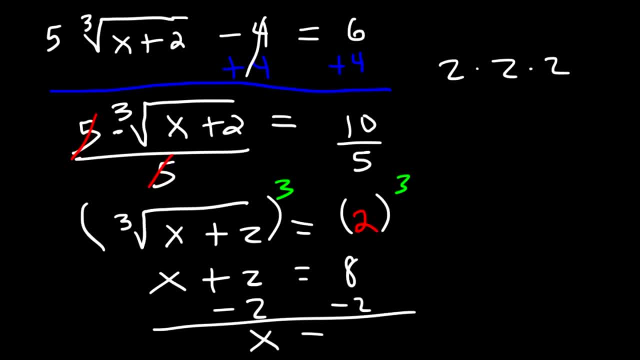 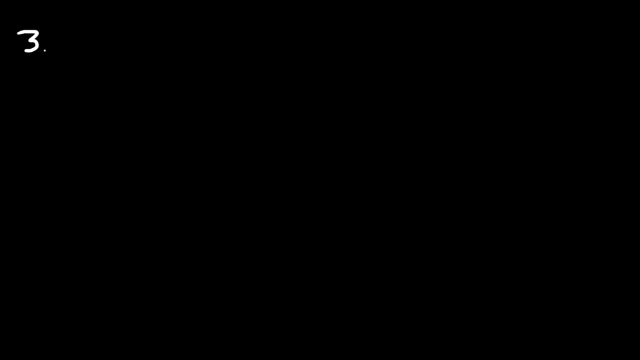 So now the last thing we need to do is subtract both sides by 2, and we'll get the final answer: x is equal to 6.. Now, what about this one? 3 times 2x minus 4,, raised to the 2 over 3, plus 5.. 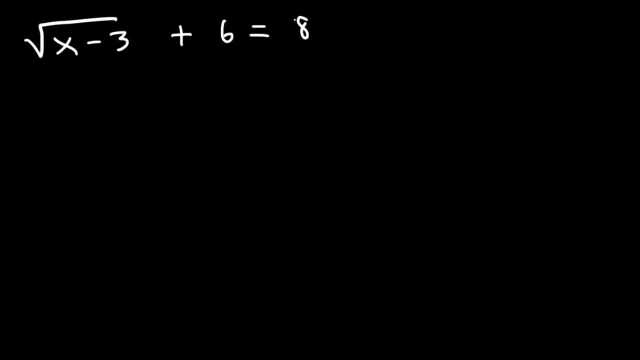 So what can we do in order to solve the variable x? Feel free to pause the video and work on the example. Well, the first thing we should do is subtract both sides by 6.. These two will cancel, and 8 minus 6 is equal to 2.. 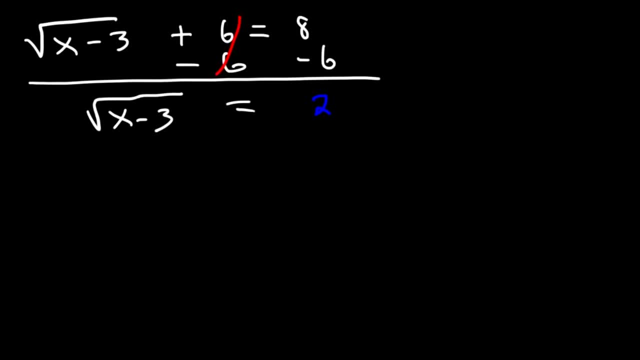 Now, what do you think we need to do at this point? How can we get rid of the square root? In order to get rid of the square root, we need to take the square of both sides. The square. The square of the square root will cancel. The index number is a 2, so these two will cancel. 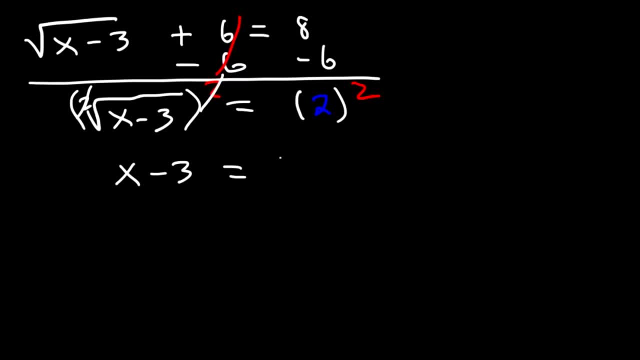 And so you're going to get: x minus 3 is equal to 2 squared, which is 4.. And now we can add 3 to both sides. 4 plus 3 is 7, so x is equal to 7.. This is the answer. 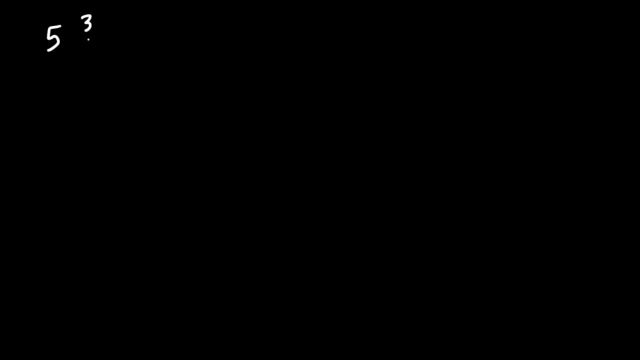 Let's try this one: 5 multiplied by the cube root of x plus 2.. Minus 4 is equal to 6.. For each of these problems, take a minute, pause the video and work on it. Try to solve it yourself first, and then see if you have the right answer. 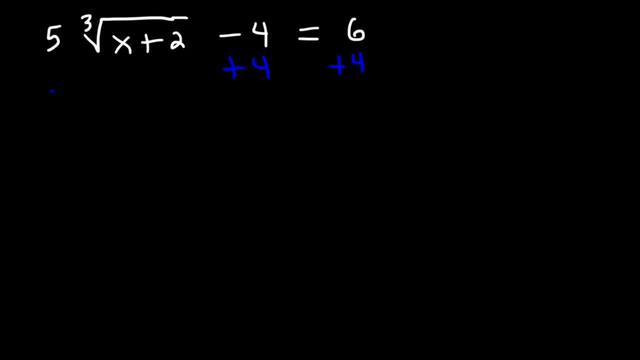 Now let's add 4 to both sides. 6 plus 4 is 10.. So 5 times the cube root of x plus 2, this is equal to 10.. So now, what do you think we need to do at this point? 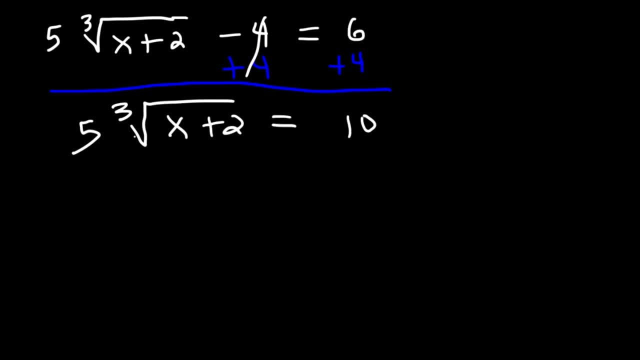 In order to separate The 5 and the cube root expression, since they're multiplied, we need to do the opposite of multiplication, which is division. 10 divided by 5 is equal to 2.. And so now we have this expression. 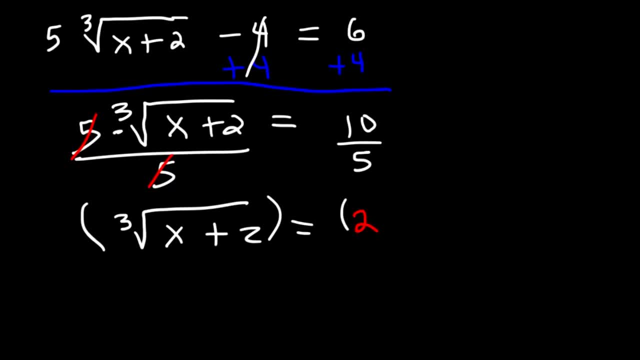 And in order to get rid of the cube root we need to raise both sides to the third power. So on the left we have x plus 2.. Now 2 to the third power is basically 2 times 2 times 2, 3 times, which is 8.. 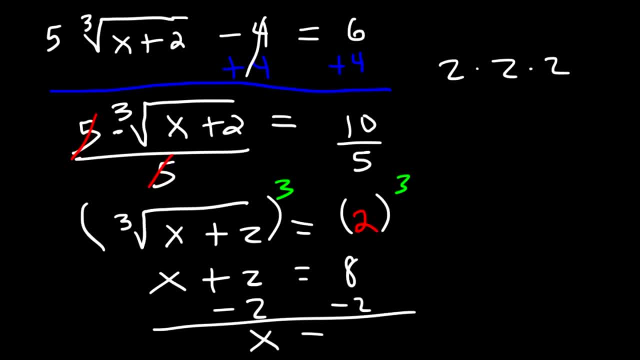 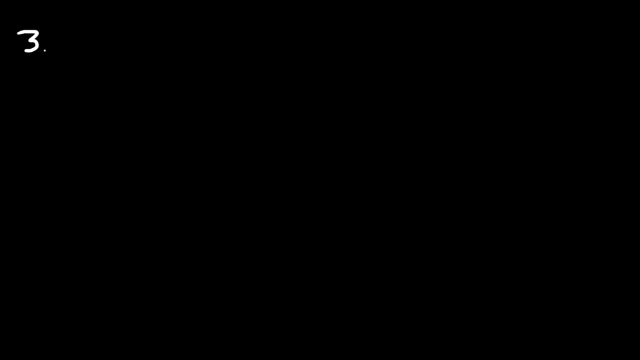 So now the last thing we need to do is subtract both sides by 2, and we'll get the final answer: x is equal to 6.. Now, what about this one? 3 times 2x minus 4,, raised to the 2 over 3, plus 5.. 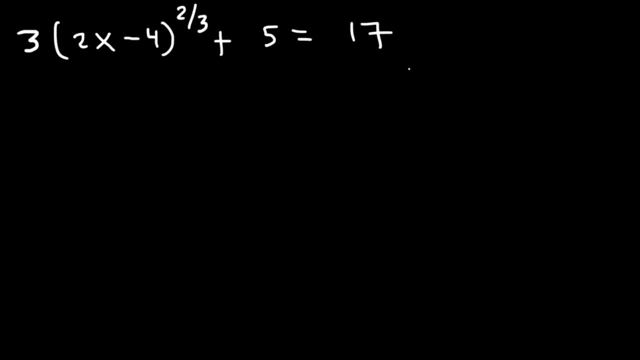 Let's say that's equal to 17.. What can we do in order to solve for x? Well, the first thing we should do is the opposite of addition, which is subtraction. 17 minus 5 is 12.. Now, in the next step, we're going to have to divide both sides by 3.. 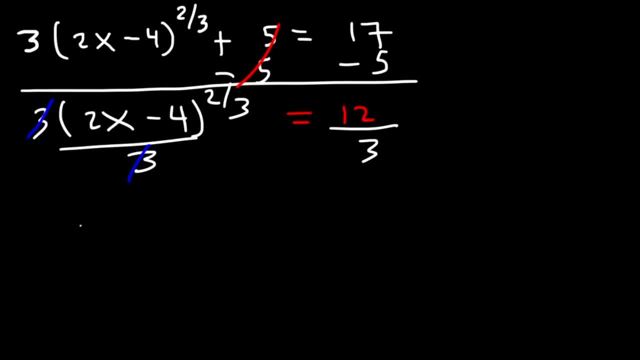 And so these two will cancel. 12 divided by 3 is 4.. Now how can we get rid of the parentheses? What should we do if we have a rational exponent? If you see something like this, raise both sides to the reciprocal of 2 over 3.. 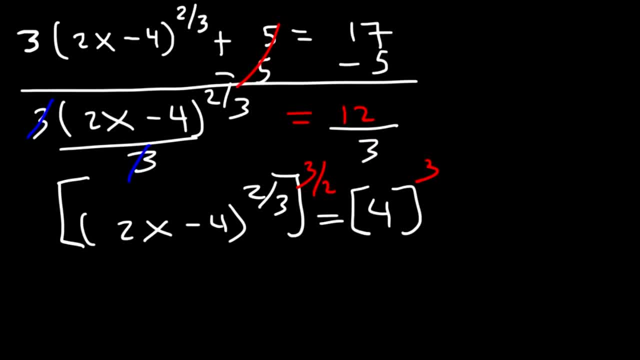 And the reciprocal is 3 over 2.. Now the reason why you want to do this is so that the 2s will cancel and the 3s will cancel, And the 3s will cancel And the 3s will cancel. 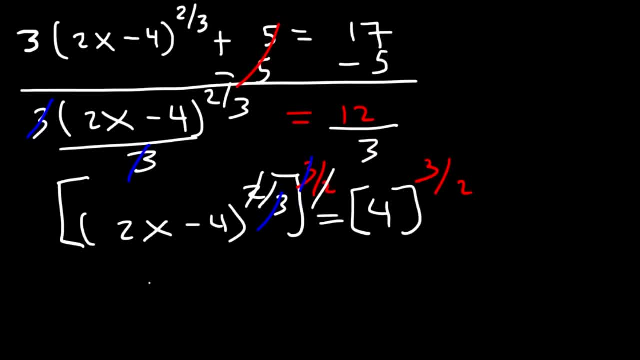 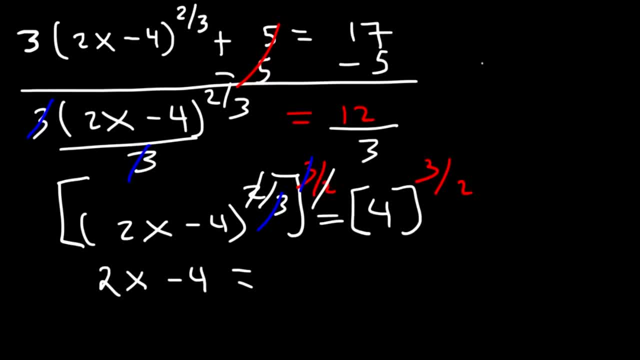 You just have 2x minus 4.. Now we need to figure out what 4 raised to the 3 halves is equal to. You can use a calculator, but if you want to do it mentally, split the fraction into two parts. 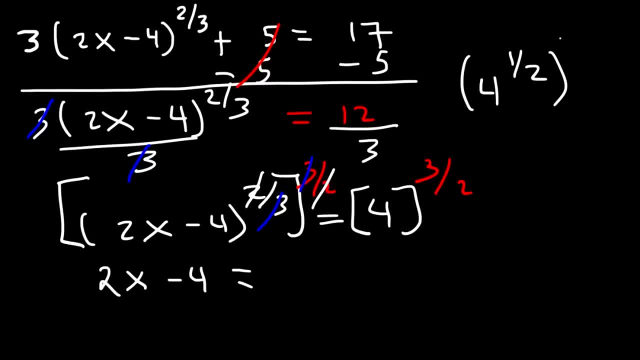 3 over 2 is basically 1 half times 3.. 4 raised to the 1 half is the same as the square root of 4, and that's 2.. 2 to the 3rd power is 8.. 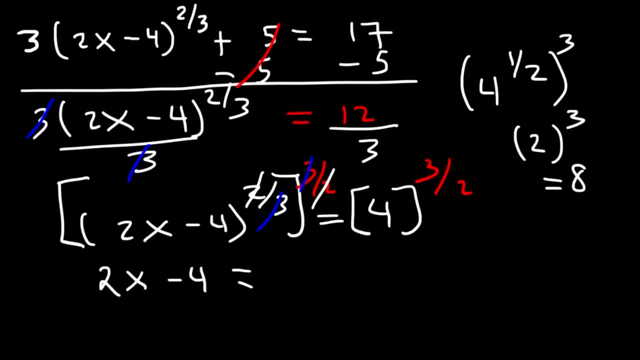 So 4 raised to the 1.5, or 3 over 2, is 8.. So now let's add 4 to both sides, So 2x is equal to 12.. And then divide both sides by 2.. 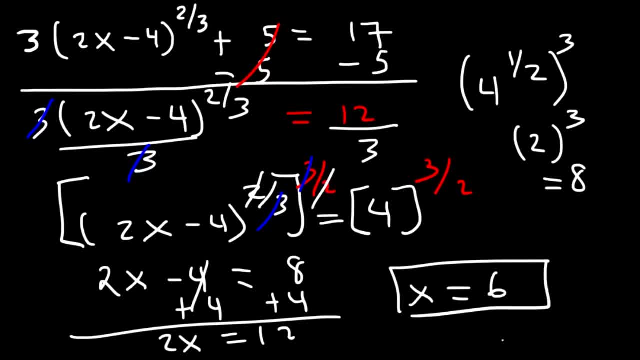 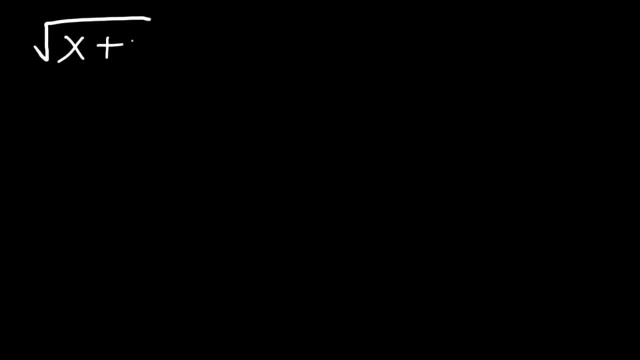 12 divided by 2 is 6.. And that's it. Try this problem. Let's say that the square root of x plus 1 is equal to 2x Minus 13. Go ahead and solve this equation. So to get rid of the square root, we need to square both sides. 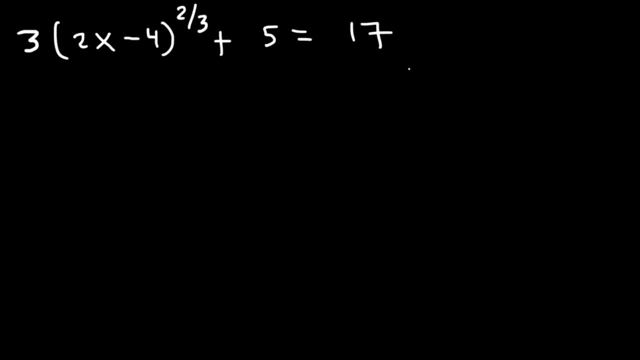 Let's say that's equal to 17.. What can we do in order to solve for x? Well, the first thing we should do is the opposite of addition, which is subtraction. 17 minus 5 is 12.. Now, in the next step, we're going to have to divide both sides by 3.. 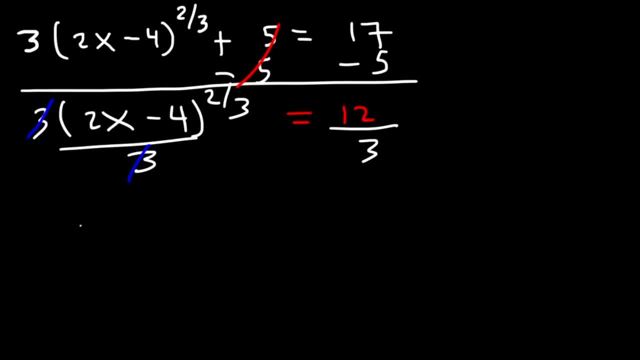 And so these two will cancel. 12 divided by 3 is 4.. Now how can we get rid of the parentheses? What should we do if we have a rational exponent? If you see something like this, raise both sides to the reciprocal of 2 over 3.. 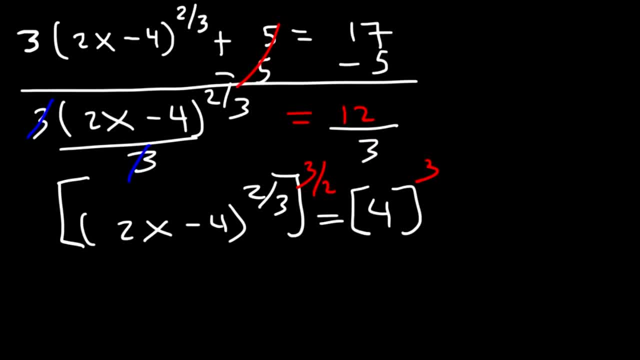 And the reciprocal is 3 over 2.. Now the reason why you want to do this is so that the 2s will cancel and the 3s will cancel, And the 3s will cancel And the 3s will cancel. 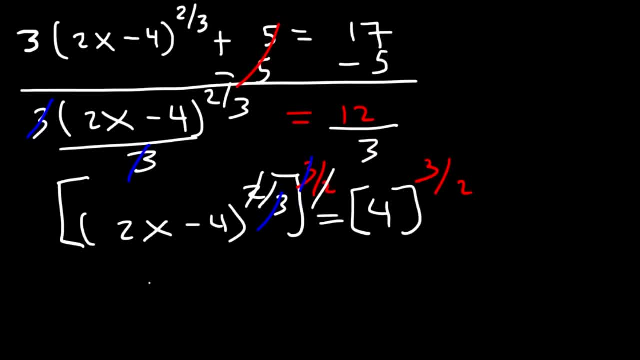 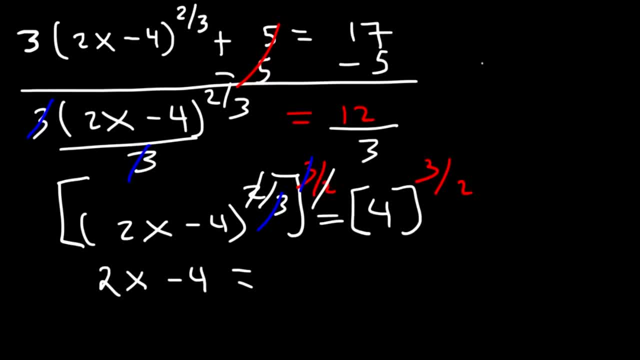 You just have 2x minus 4.. Now we need to figure out what 4 raised to the 3 halves is equal to. You can use a calculator, but if you want to do it mentally, split the fraction into two parts. 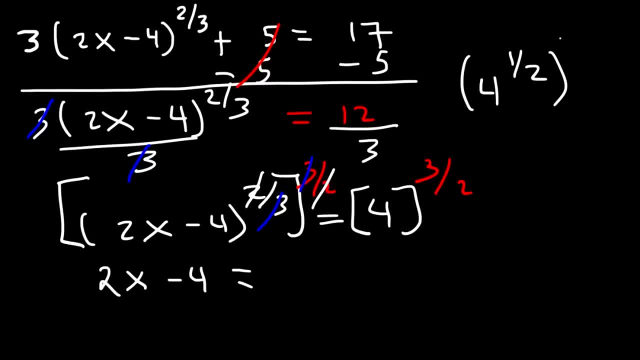 3 over 2 is basically 1 half times 3.. 4 raised to the 1 half is the same as the square root of 4, and that's 2.. 2 to the 3rd power is 8.. 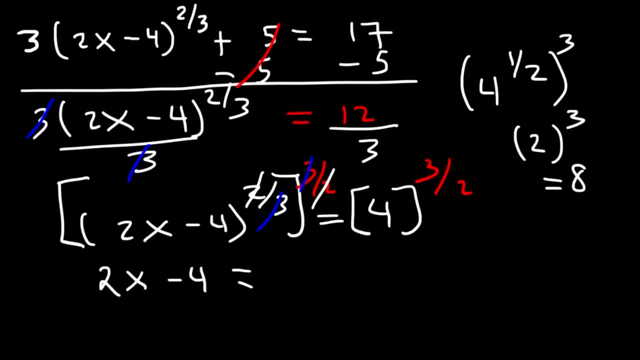 So 4 raised to the 1.5, or 3 over 2, is 8.. So now let's add 4 to both sides, So 2x is equal to 12.. And then divide both sides by 2.. 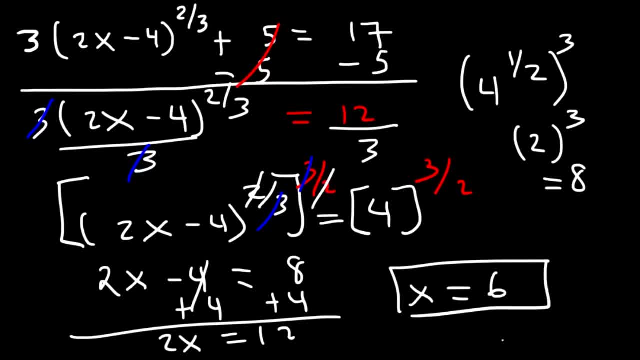 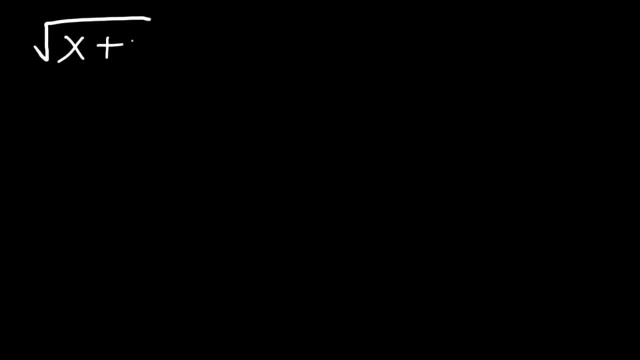 12 divided by 2 is 6.. And that's it. Try this problem. Let's say that the square root of x plus 1 is equal to 2x Minus 13. Go ahead and solve this equation. So to get rid of the square root, we need to square both sides. 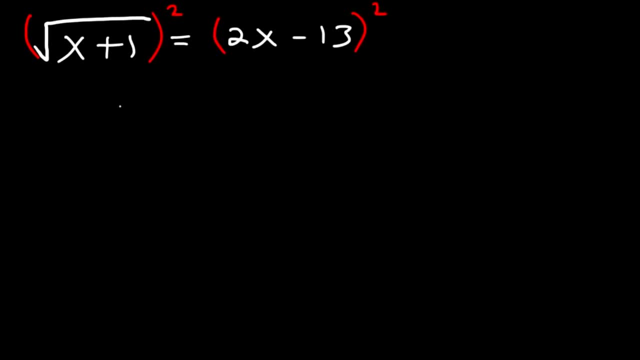 That's the first thing we need to do. So on the left side we have x plus 1.. But on the right side we need to FOIL 2x minus 13.. 2x minus 13 squared is 2x minus 13 times another 2x minus 13.. 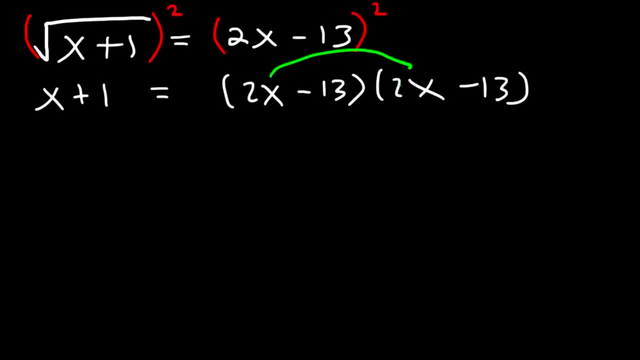 So we have two of them Now. 2x times 2x is 4x squared. 2x times negative: 13 is negative 26x. Negative 13 times 2x is also negative 26x And negative 13 times negative, 13 is positive 169.. 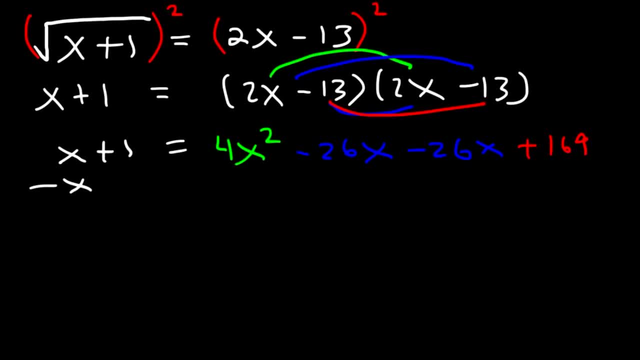 So now we're going to subtract both sides by x. Well, actually, before we do that, let's combine like terms. So if we combine those two, it's going to be negative 52x. And now let's subtract both sides by x and 1.. 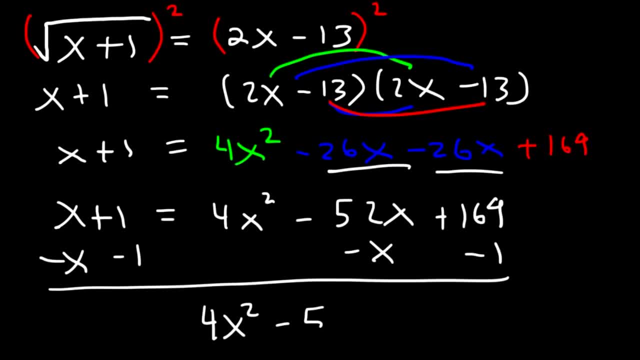 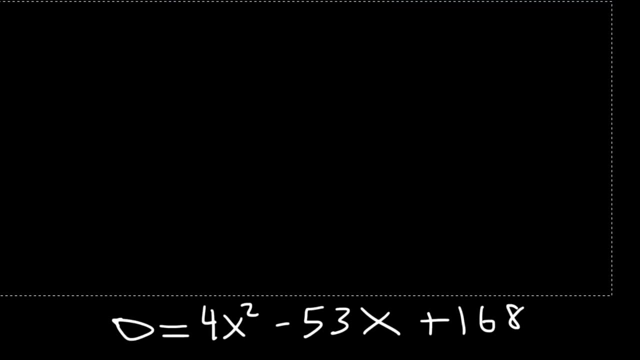 So we're going to have 4x squared minus 53x plus 168.. And this is equal to 0.. So now, at this point, what we can do is we could try to factor the expression, or we can use the quadratic equation to solve it. 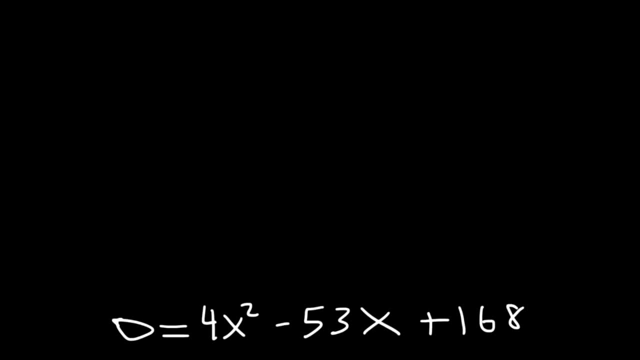 I think it's easier to use the quadratic equation. Let's say: if you want to factor it, You need to multiply 4 and 168.. 4 times 168 is 672.. So you've got to find two numbers that multiply to 672. 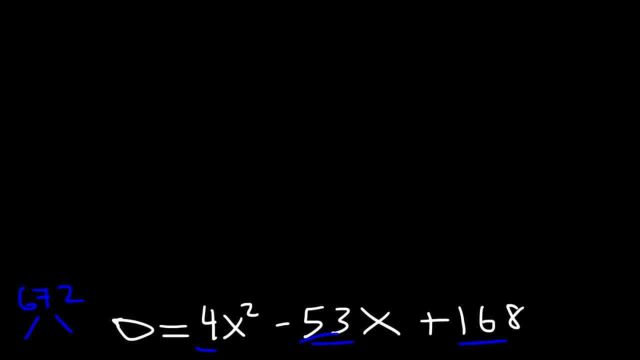 but that add to the middle coefficient negative 53. And that's going to take a lot of work. So, using the quadratic formula, a is 4, b is negative 53, c is 168.. So here's the formula. 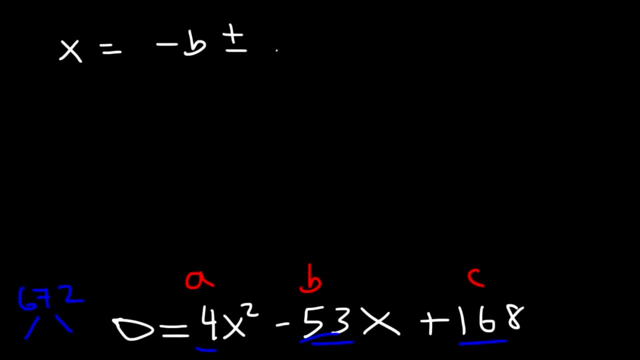 It's x is equal to negative b plus or minus the square root of b squared minus 4ac divided by 2a. So b is negative 53. That means b squared, That's 53 squared. Once you square it, it's no longer going to be negative. 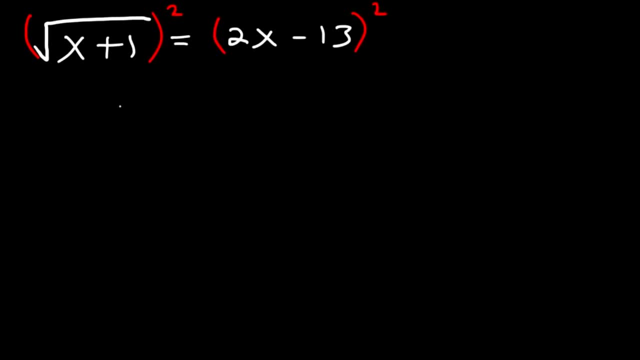 That's the first thing we need to do. So on the left side we have x plus 1.. But on the right side we need to FOIL 2x minus 13.. 2x minus 13 squared is 2x minus 13 times another 2x minus 13.. 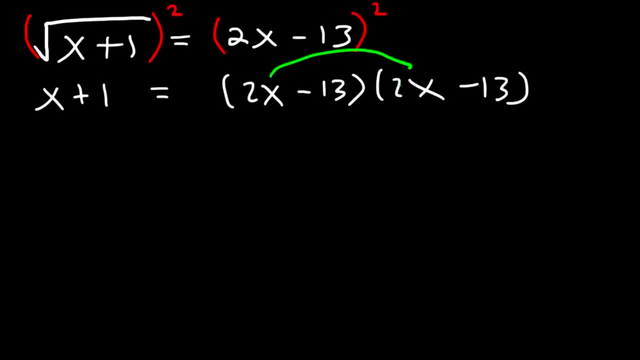 So we have two of them Now. 2x times 2x is 4x squared. 2x times negative: 13 is negative 26x. Negative 13 times 2x is also negative 26x And negative 13 times negative, 13 is positive 169.. 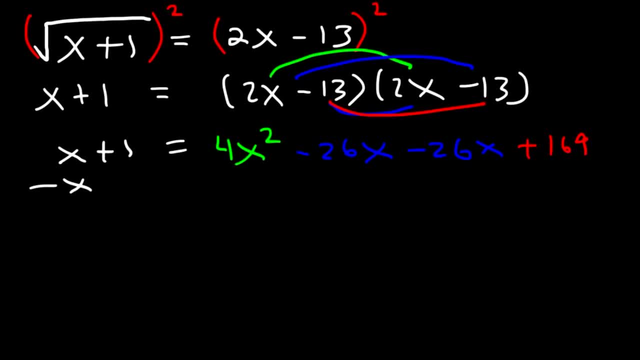 So now we're going to subtract both sides by x. Well, actually, before we do that, let's combine like terms. So if we combine those two, it's going to be negative 52x. And now let's subtract both sides by x and 1.. 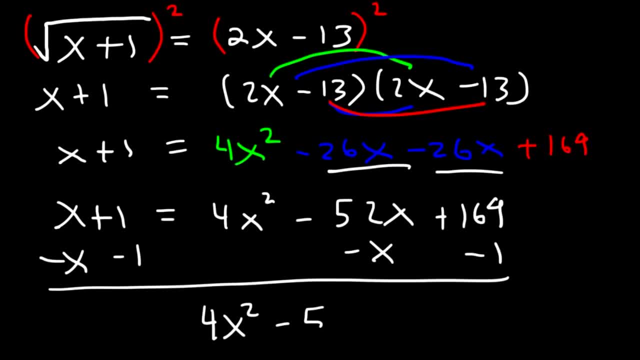 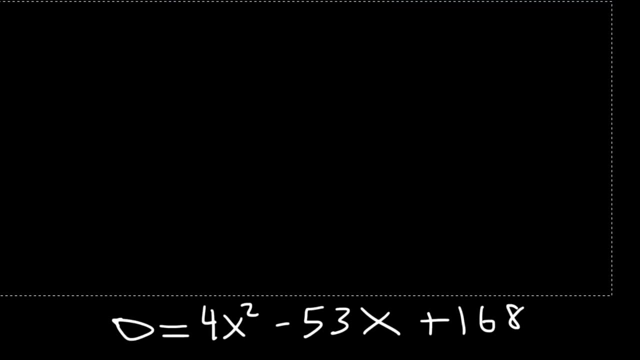 So we're going to have 4x squared minus 53x plus 168.. And this is equal to 0.. So now, at this point, what we can do is we could try to factor the expression, or we can use the quadratic equation to solve it. 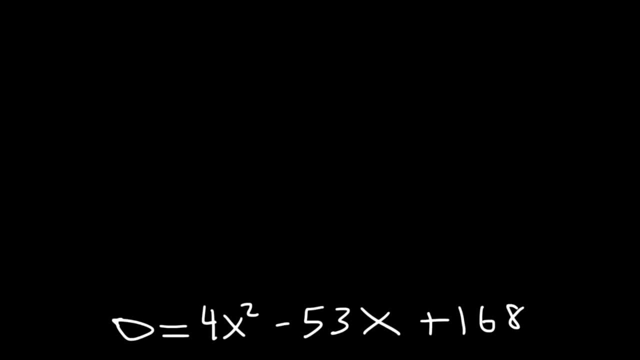 I think it's easier to use the quadratic equation. Let's say: if you want to factor it, You need to multiply 4 and 168.. 4 times 168 is 672.. So you've got to find two numbers that multiply to 672,. 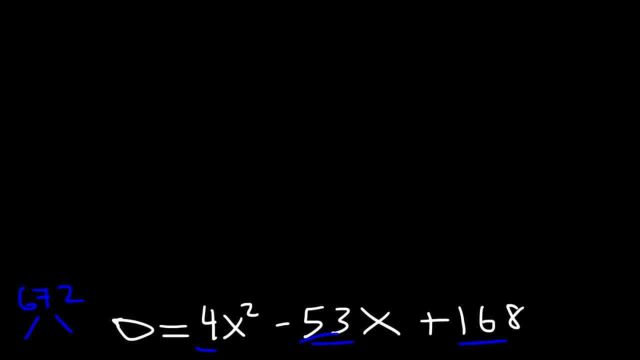 but that add to the middle coefficient negative 53. And that's going to take a lot of work. So, using the quadratic formula, a is 4, b is negative 53, c is 168.. So here's the formula. 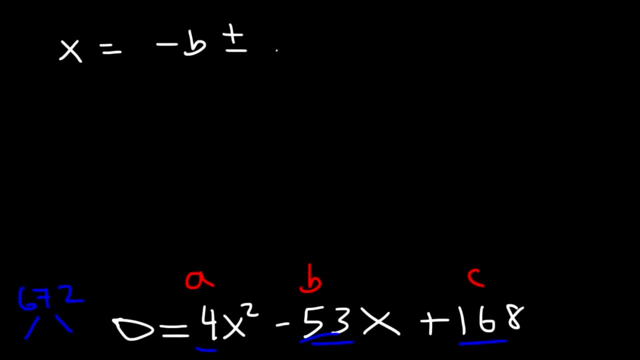 It's x is equal to negative b plus or minus the square root of b squared minus 4ac divided by 2a. So b is negative 53. That means b squared, That's 53 squared. Once you square it, it's no longer going to be negative. 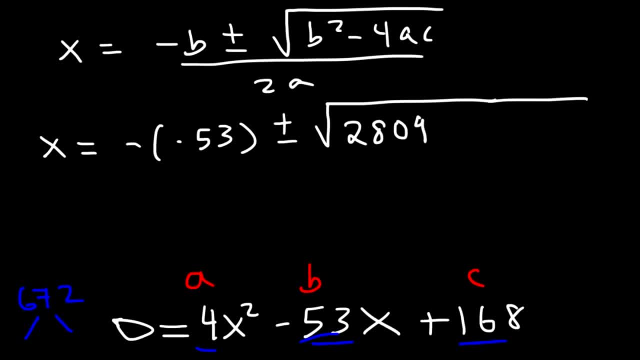 It's going to be positive, And it's 2809.. a is 4, and c is 168.. And all of this is divided by 2a, which is 2 times 4, and that's 8.. So now we have positive 53,, 2809.. 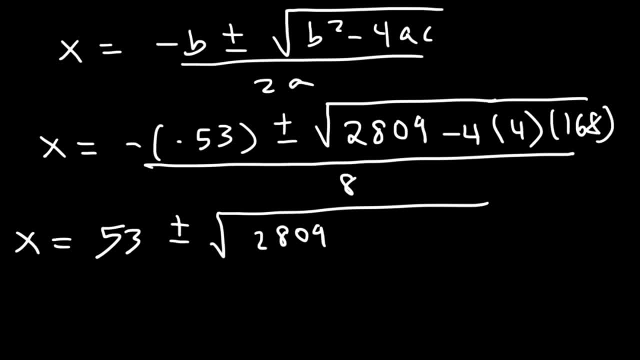 Negative 4 times 4 is negative 16, and multiply it by 168.. That's negative 2688.. 2809 minus 2688.. 2809 minus 2688.. is 121.. The square root of 121 is: 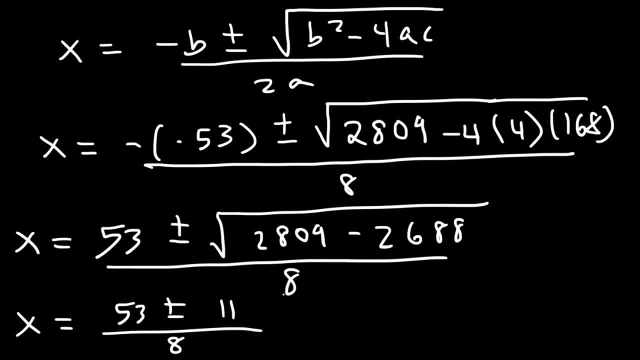 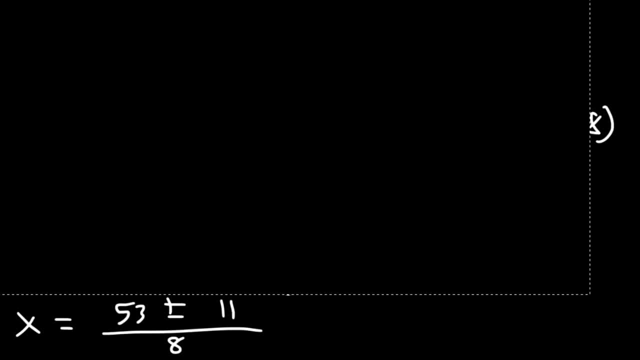 11.. So now we have two possible answers. Those two possible answers are: 53 plus 11 divided by 8, and 53 minus 11 divided by 8.. 53 plus 11 is 64.. And 53 minus 11, that's 42.. 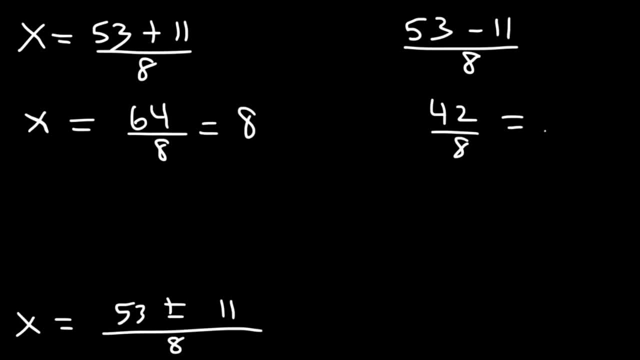 64 divided by 8 is 8.. 42 divided by 8, we can reduce that. If we divide both numbers by 2, it's going to be 21 over 4.. Which, as a decimal that's 5.25.. 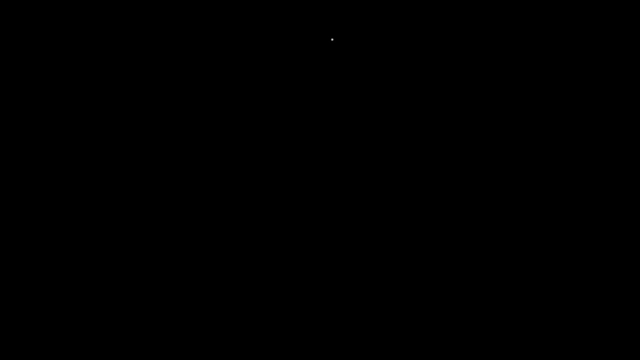 So now let's check the answers. So we have: x is equal to 8 or 5.25.. Now the original equation was square root: x plus 1, and that's equal to 2x minus 13.. Since we have, 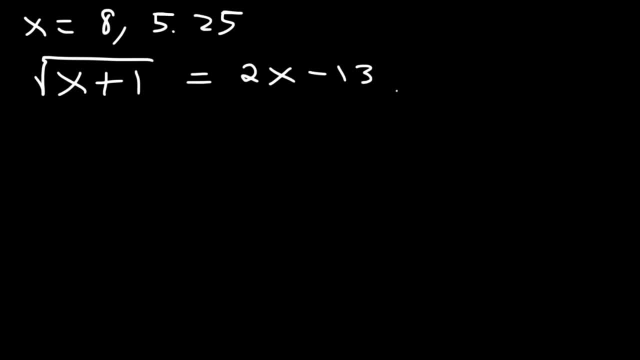 two answers. we've got to check to see if one of them is an extraneous solution. So let's try 8.. 8 plus 1 is 9.. 2 times 8 is 16.. The square root of 9 is 3.. 16 minus 13 is 3.. 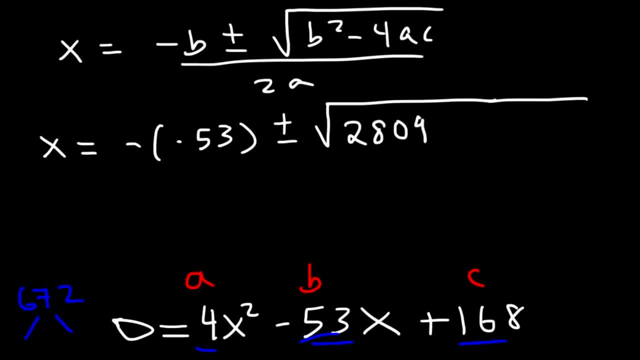 It's going to be positive, And it's 2809.. a is 4 and c is 168.. And all of this is divided by 2a, which is 2 times 4. And that's 8.. So now we have positive 53,, 2809.. 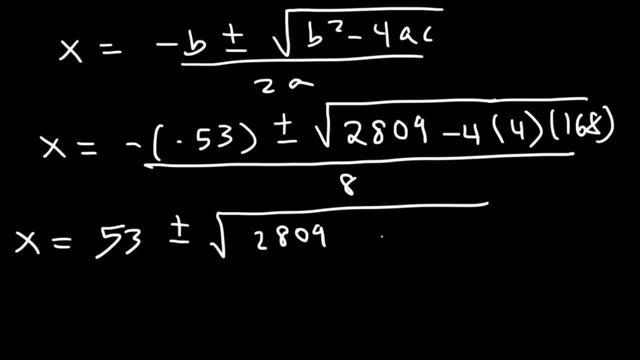 Negative. 4 times 4 is negative 16. And multiply it by 168.. That's negative 2688.. 2809 minus 2688.. 2809 minus 2688.. 2809 minus 2688 is 121.. 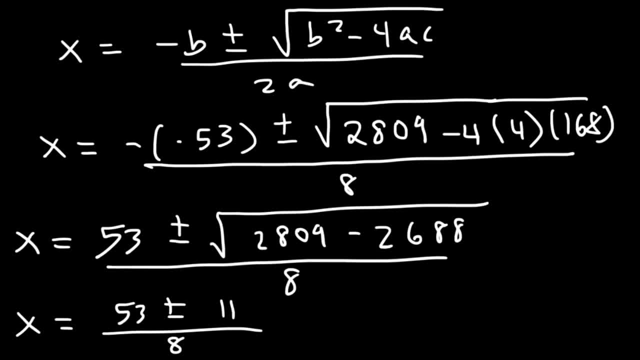 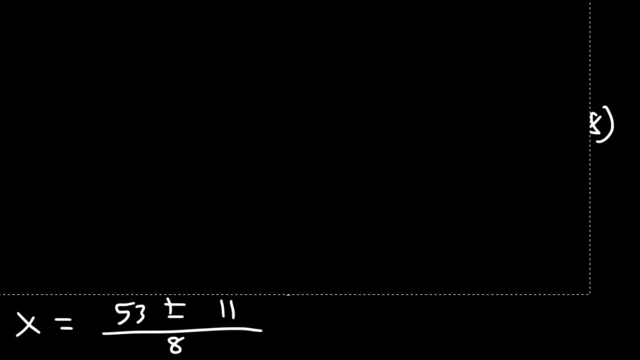 The square root of 121 is 11.. So now we have two possible answers. Those two possible answers are 53 plus 11.. 11 divided by 8. And 53 minus 11 divided by 8.. 53 plus 11 is 64.. 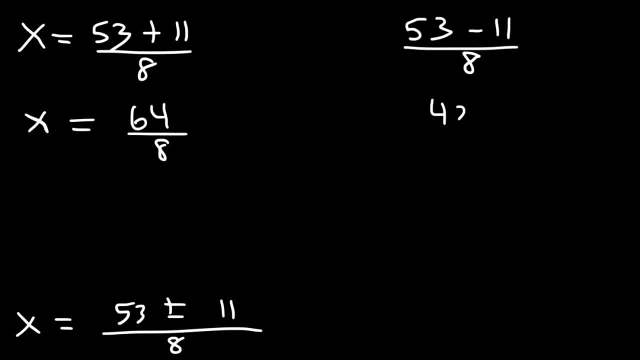 And 53 minus 11, that's 42.. 64 divided by 8 is 8.. 42 divided by 8, we can reduce that. If we divide both numbers by 2, it's going to be 21 over 4.. 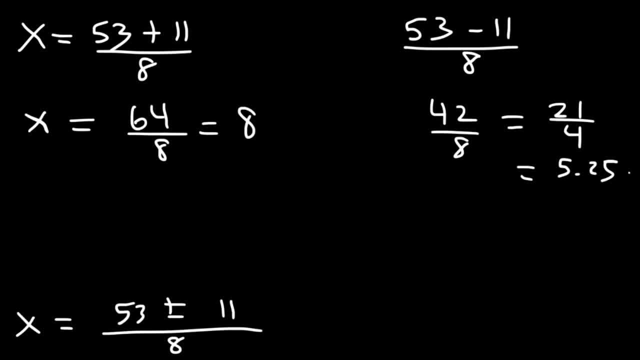 Which, as a decimal, that's 5.25.. So now let's check the answers. So we have: x is equal to 8 or 5.25.. Now the original equation was square root x plus 1.. And that's equal to 2x minus 13.. 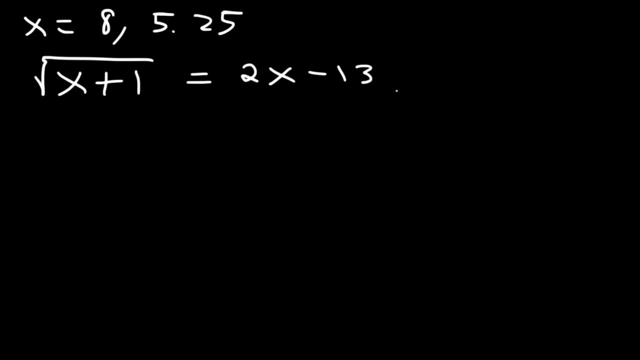 Since we have two answers, we've got to check to see if one of them is an extraneous solution. So let's try 8.. 8 plus 1 is 9.. 2 times 8 is 16.. The square root of 9 is 3.. 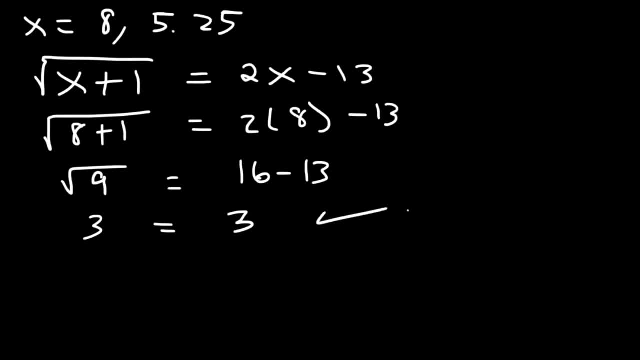 16 minus 13 is 3.. So that works. Now let's try the other answer. Let's try 5.25.. 5.25., 5.25., 5.25., 5.25.. 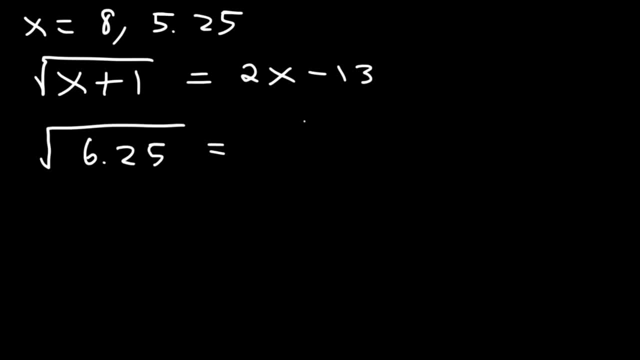 Plus 1 is 6.25.. 2 times 5.25 is 10.5.. Now the square root of 6.25 is positive 2.5.. And 10.5 minus 13 is negative 2.5.. 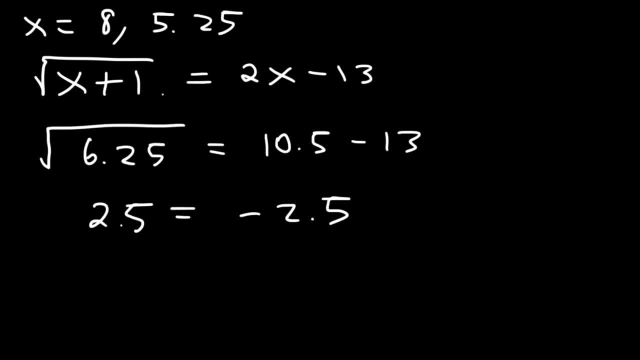 So this doesn't work. Therefore, we can say that the other answer is an extraneous solution. So the answer is: x is equal to 8.. Now let's try a problem where we have two radicals. In a situation like this, what do you think we should do? 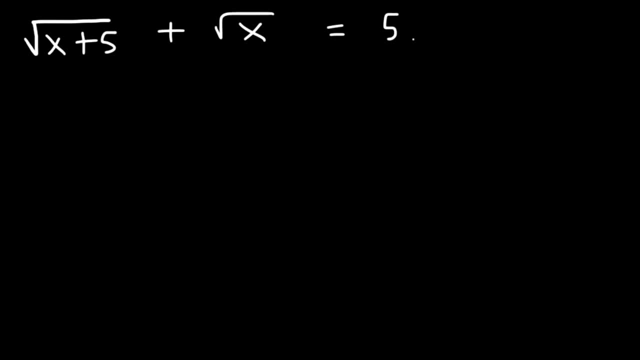 How can we even solve this thing If you have two radicals? what you want to do is you want to put one of the radicals on one side and the other on the other side. Make sure they're on different sides. So let's move the square root x from the left side to the right side. 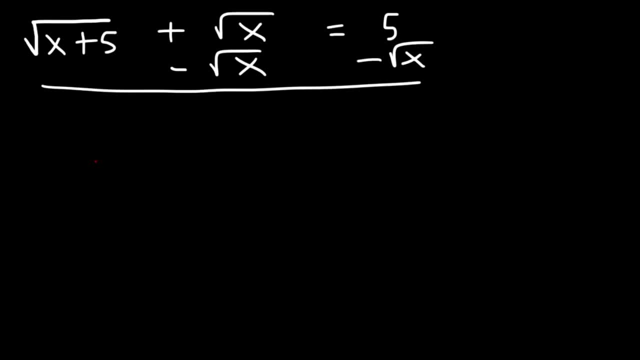 It's positive on the left side, but it's going to be negative on the right side. So what we have now is this expression. So now what we need to do is take the square of both sides. On the left side, the square root will disappear. 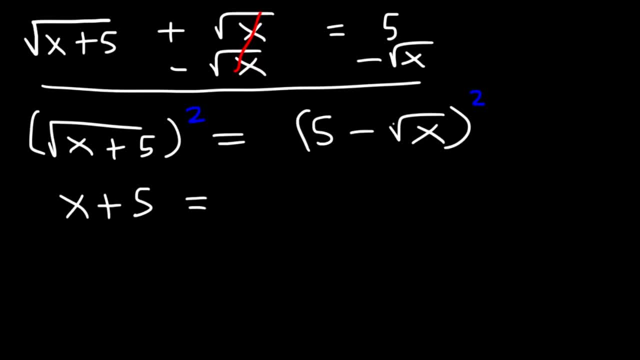 We're just going to get x plus 5. On the right side, because the 5 and the square root are separated by a negative sign, you have to FOIL. You're going to have to write it twice and FOIL this expression. 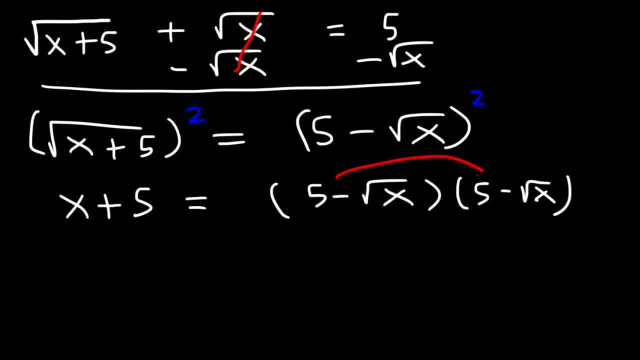 There's no way around this. Now, 5 times 5 is 25.. 5 times negative root x is negative. 5 root x. This part is also negative. 5 root x: Negative 5 root x. Negative square root x. 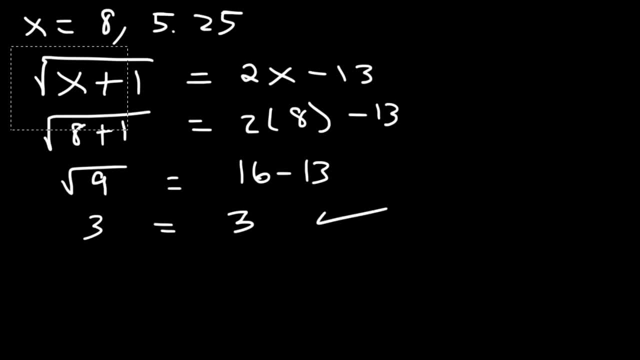 So that works. Now let's try the other answer. Let's try 4.. 5.25.. 5.25 plus 1 is 6.25.. 2 times 5.25 is 10.5.. 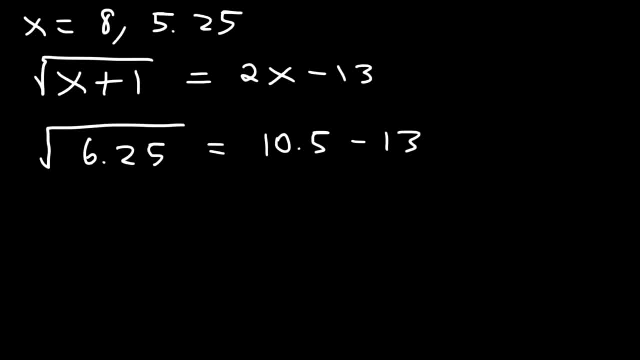 Now the square root of 6.25 is positive 2.5. And 10.5 minus 13 is negative 2.5. So this doesn't work. Therefore, we can say that the other answer is an extraneous solution. 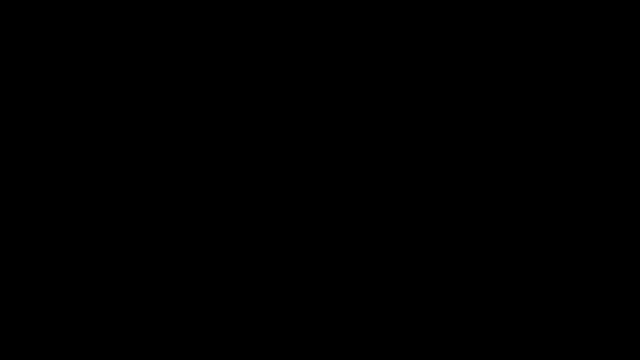 So the answer is: x is equal to 8.. Now let's try a problem where we have two radicals. In a situation like this, what do you think we should do? How can we even solve this thing If you have two radicals? what you want to do is you want to put one of the radicals. 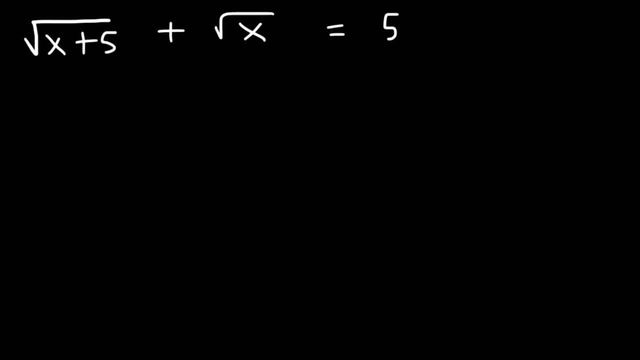 on one side and the other on the other side. Make sure they're on different sides. So let's move the square root x from the left side to the right side. It's positive on the left side, but it's going to be negative on the right side. 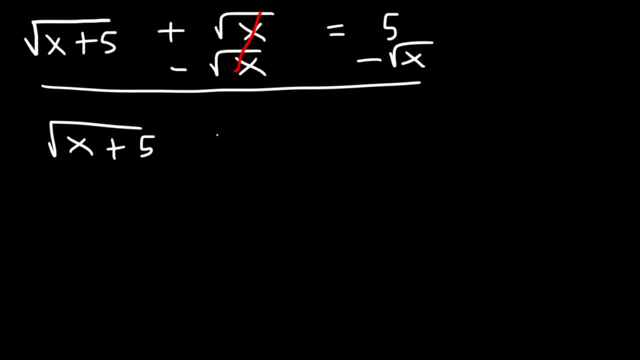 So what we have now is this expression. So now what we need to do is take the square of both sides. On the left side, the square root will disappear. We're just going to get x. We're just going to get x plus 5.. 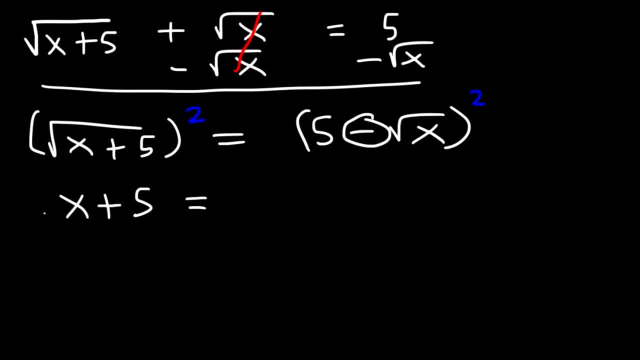 On the right side, because the 5 and the square root are separated by a negative sign. you have to FOIL. You're going to have to write it twice and FOIL this expression. There's no way around this. Now, 5 times 5 is 25.. 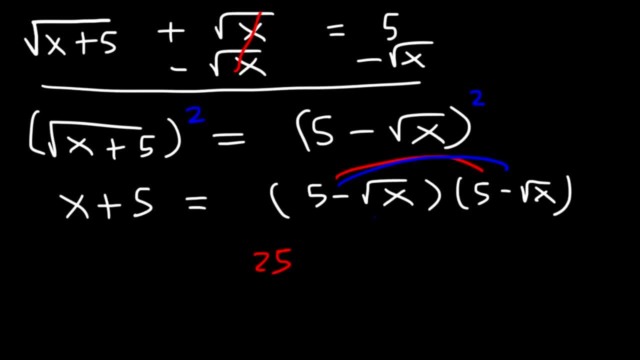 5 times negative root x is negative 5 root x- This part is also negative 5 root x. Negative square root: x times negative square root x is simply positive x. Two negatives will make a positive And on this side we just have x plus 5.. 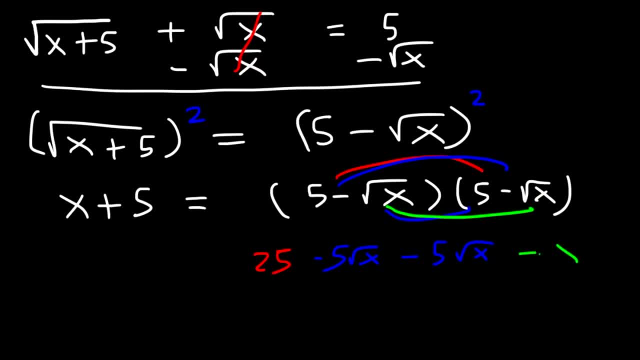 Negative square root x times negative square root x is simply positive x. Two negatives will make a positive, And on this side we just have x plus 5.. So now, if we combine like terms, this is going to be 25 minus 10 root x plus x. 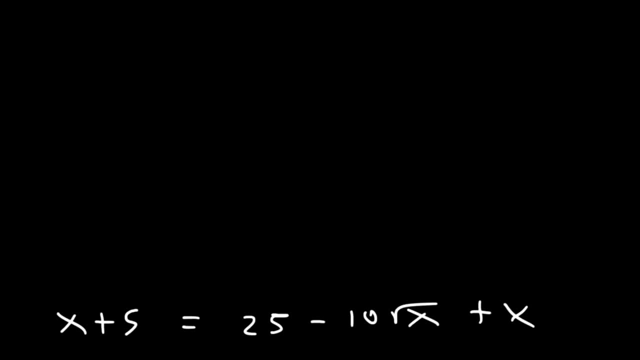 So now we have 25 minus 10 root x plus x. Now what we need to do is subtract both sides by x So that these will cancel, And so now we have: 5 is equal to 25 minus 10 root x. 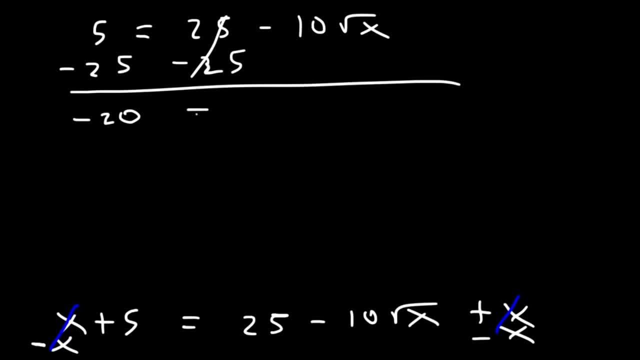 Now let's subtract both sides by 25.. 5 minus 25 is negative 20.. Let's divide both sides by negative 10.. Negative 20 divided by negative 10, that's 2.. So 2 is equal to the square root of X. 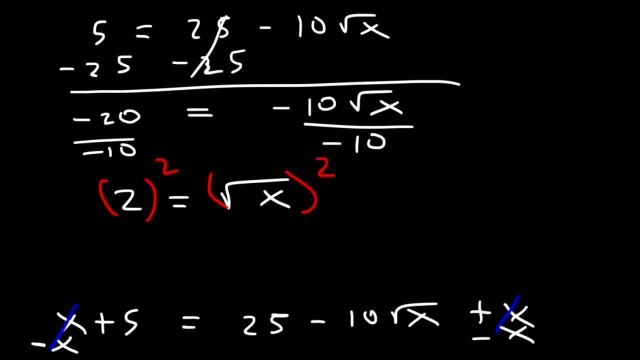 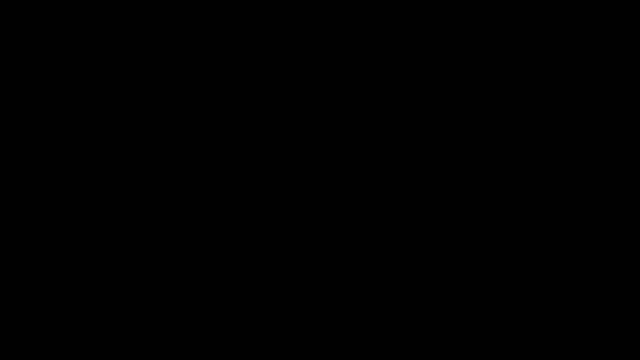 So therefore, if we square both sides, 2 squared is 4 and the square root of X squared is X. So therefore, X is equal to 4.. And just to be on the safe side, let's go ahead and make sure that the answer is correct. 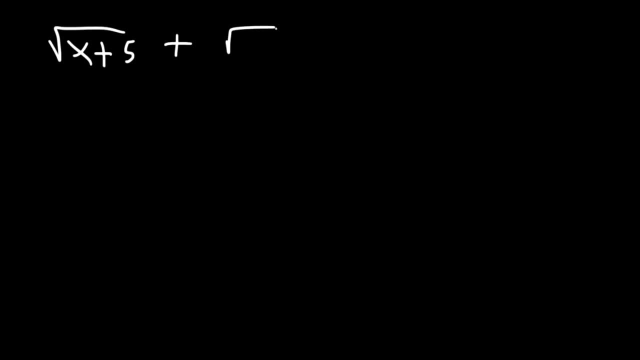 X is indeed equal to 4.. So let's plug it in. We're going to have 4 plus 5 plus the square root of 4, and that should be equal to 5.. 4 plus 5 is 9.. The square root of 4 is 2.. 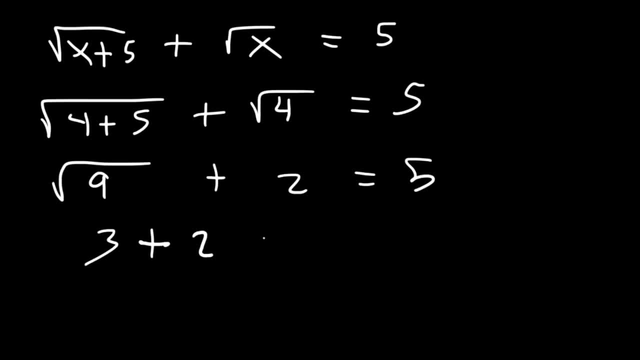 The square root of 9 is 3.. And 3 plus 2 is equal to 5.. So we know that X is indeed equal to 4.. Here's another one that you could try: The square root of X plus 8, divided by the square root of X, is equal to 6.. 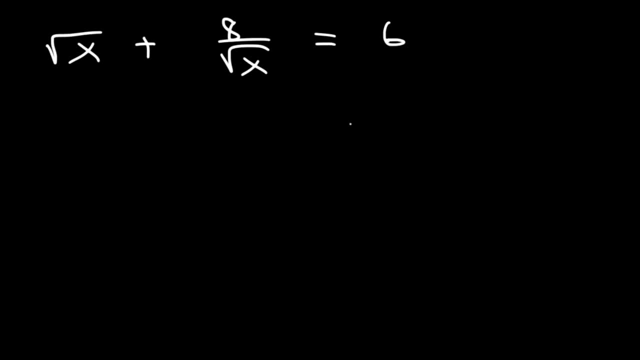 What is the value of X? So here we have a fraction. What do you think we need to do in order to get X by itself? in a situation like this, The best thing to do is to get rid of the fraction, Since the denominator contains the square root of X. multiply everything by the square. 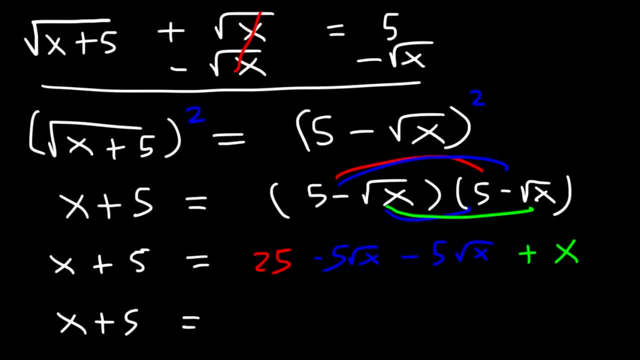 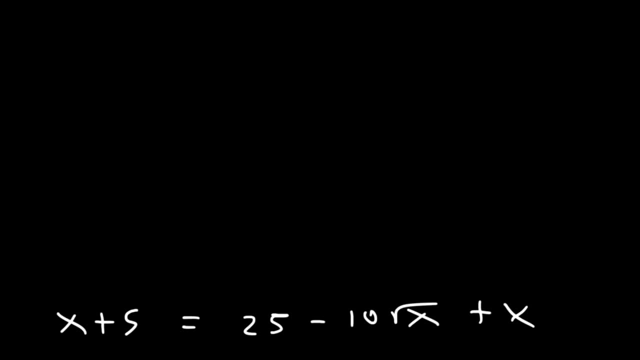 So now, if we combine like terms, this is going to be 25 minus 10 root x, times negative square root x Plus x. Now what we need to do is subtract both sides by x So that these will cancel, And so now we have: 5 is equal to 25 minus 10 root x. 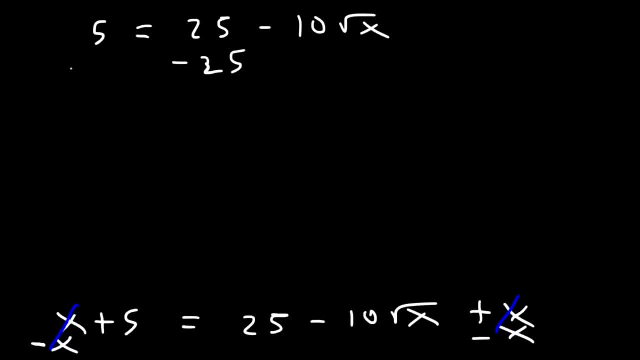 Now let's subtract both sides by 25.. 5 minus 10 root x times negative. square root x is negative 5 root x. Now what we need to do is subtract both sides by x. 5 minus 25 is negative 20.. 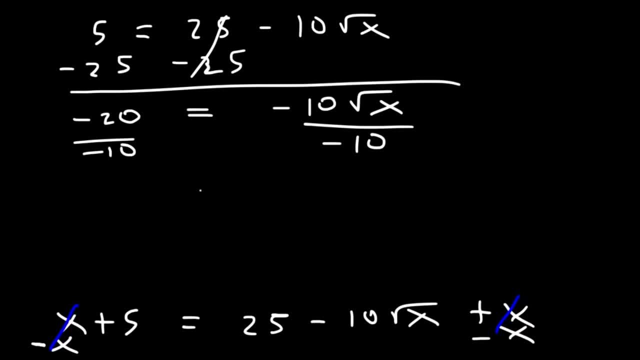 And now let's divide both sides by negative 10.. Negative 20 divided by negative 10, that's 2.. So 2 is equal to the square root of x. So therefore, if we square both sides, 2 squared is 4.. 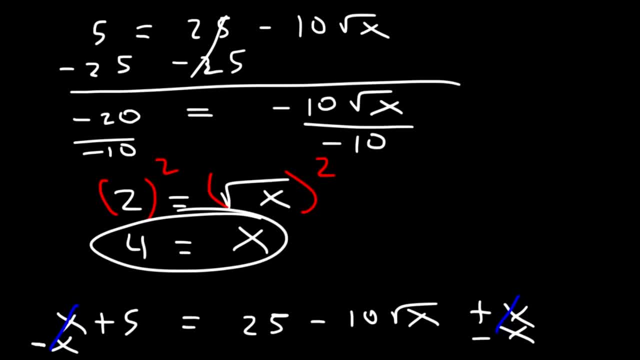 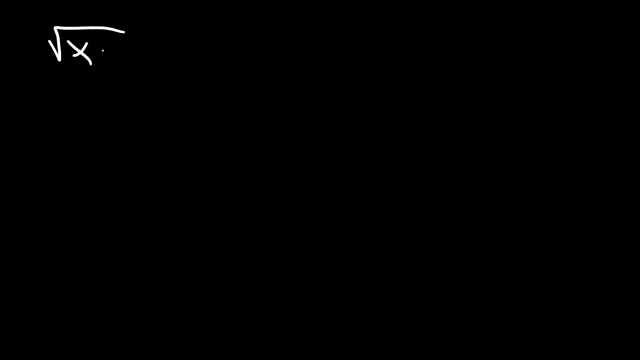 And the square root of x squared is x. So therefore x is equal to 4.. And just to be on the safe side, Let's go ahead. Let's make sure that the answer is correct: That x is indeed equal to 4.. 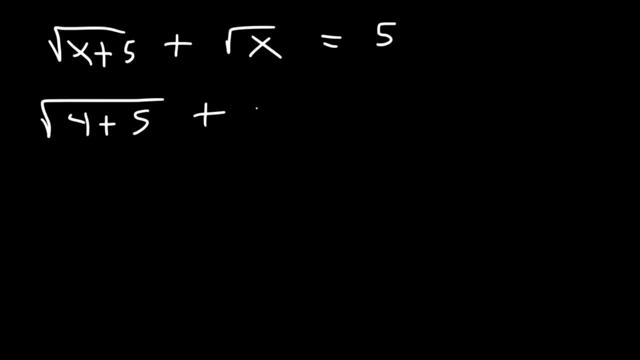 So let's plug it in. We're going to have 4 plus 5 plus the square root of 4. And that should be equal to 5.. 4 plus 5 is 9.. The square root of 4 is 2.. 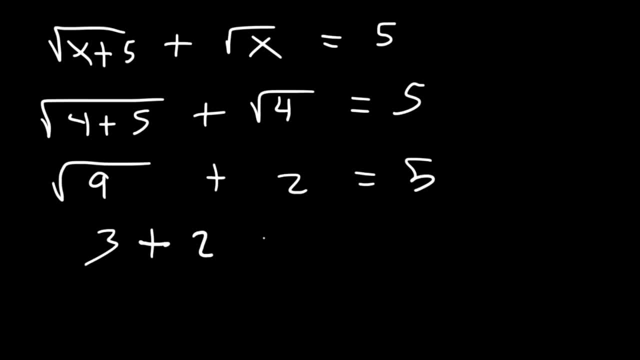 The square root of 9 is 3.. And 3 plus 2 is equal to 5.. Okay, So we know that x is indeed equal to 4.. Here's another one that you can try: The square root of x plus 8, divided by the square root of x, is equal to 6.. 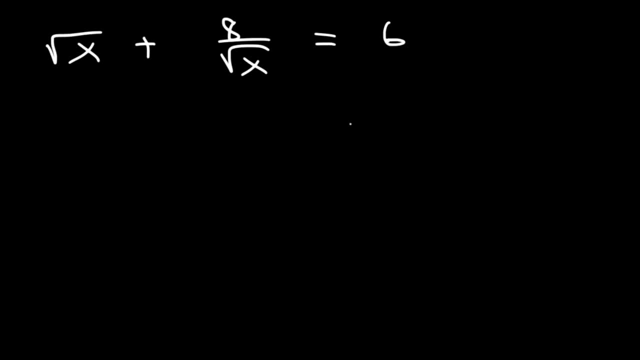 What is the value of x? So here we have a fraction. What do you think we need to do in order to get x by itself? in a situation like this, The best thing to do is to get rid of the fraction, Since the denominator contains the square root of x. 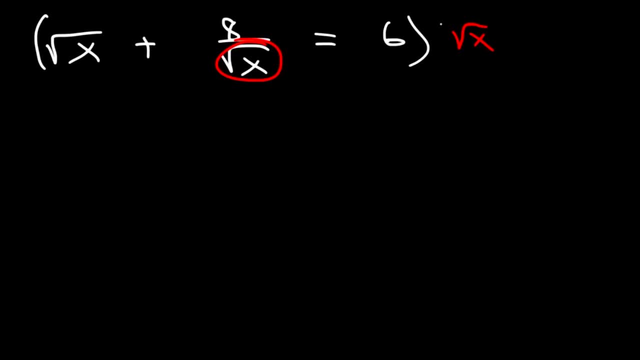 multiply everything by the square root of x. The square root of x times the square root of x is simply x, And if we multiply root x by 8 over root x, these two will cancel, giving us just 8.. And then finally, we have 6 multiplied by root x. 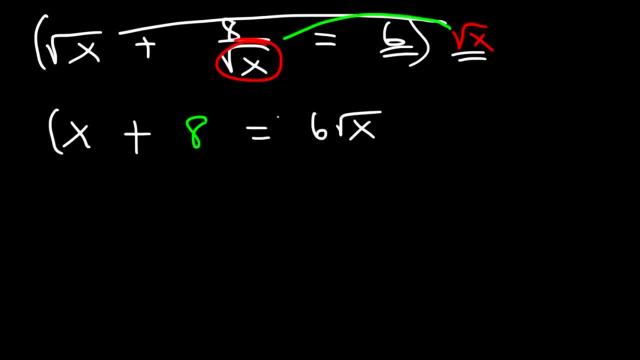 which is just 6 root x. So now, at this point, to get rid of the radical on the right side, we need to take the square of both sides. On the left side, we need to FOIL x plus 8 times x plus 8.. 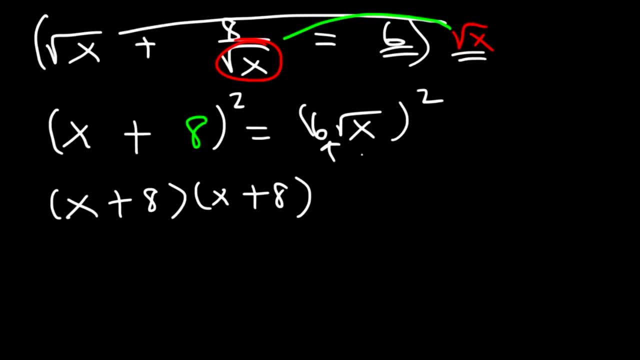 On the right side. we don't have to. We don't have a plus or minus sign that separates the 6 and the square root x, Because they're multiplied. we can square the 6,, which is 36,, and the square of root x is simply x, so we get 36x. 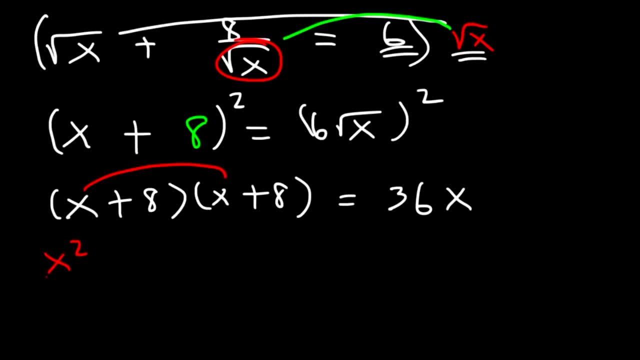 But now let's FOIL: x times x is x squared x times 8. is 8x, and this is also 8x. And then 8 times 8 is 64.. So, combining like terms, we have x squared plus 16x plus 64.. 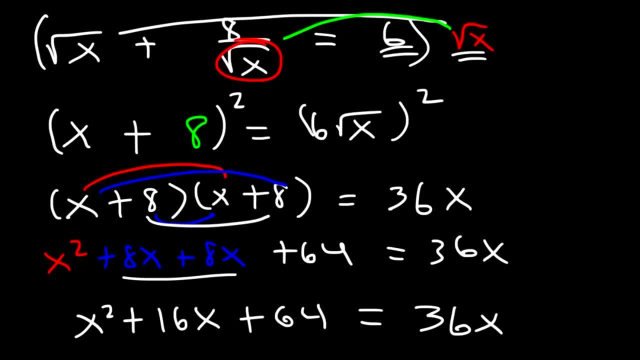 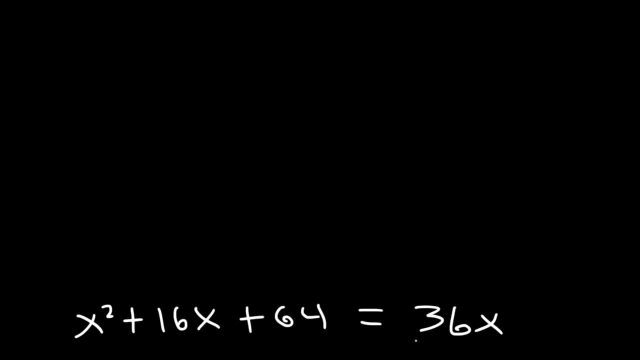 All of that is equal to 36x. Now let's subtract both sides by 36x, So we get 16x minus 36.. 16 minus 36 is negative 20.. So here we have a trinomial with a leading coefficient of 1.. 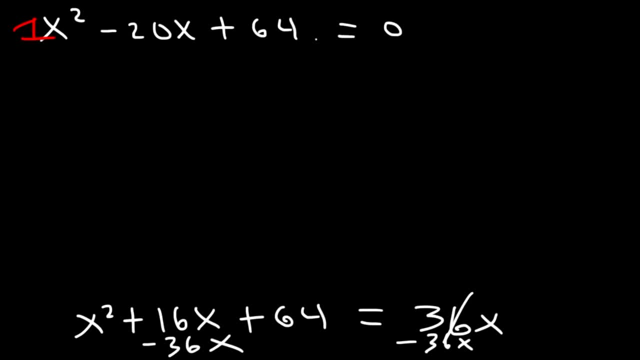 Now, in order to factor this trinomial, we need to find two numbers that multiply to 64, but add to negative 20.. So what are some numbers that multiply to 64?? We have 8 and 8,, 4 and 16.. 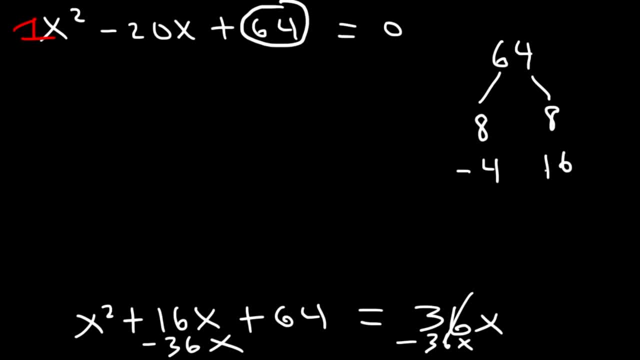 Notice that 4 plus 16, adds up to 20.. Negative 4 and negative 16 adds up to negative 20, but still multiplies to positive 64. So this is going to be x minus 4 times x minus 16.. 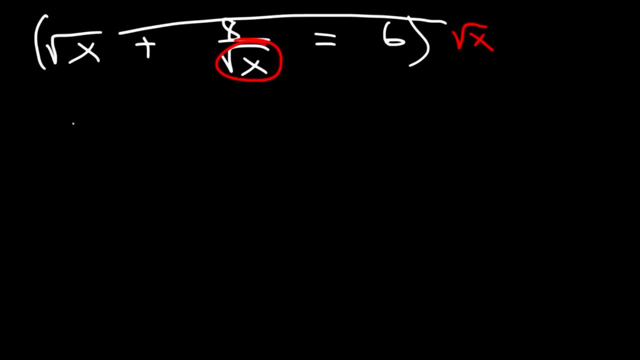 root of X. The square root of X times the square root of X is simply X, And if we multiply root X by 8 over root X, these two will cancel, giving us just 8.. And then finally we have 6 multiplied by root X, which is just 6 root X. 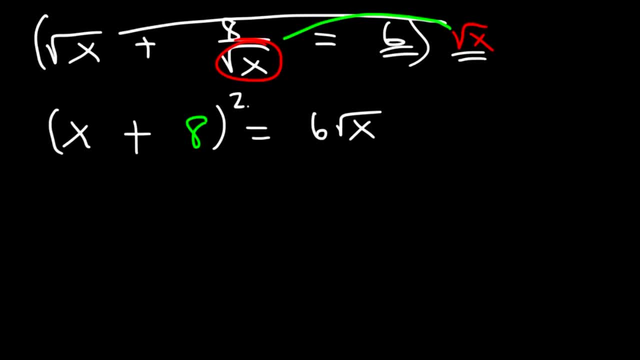 So now, at this point, to get rid of the radical on the right side, we need to take the square of both sides. On the left side, we need to FOIL X plus 8.. So what do we do? X plus 8 times X plus 8.. 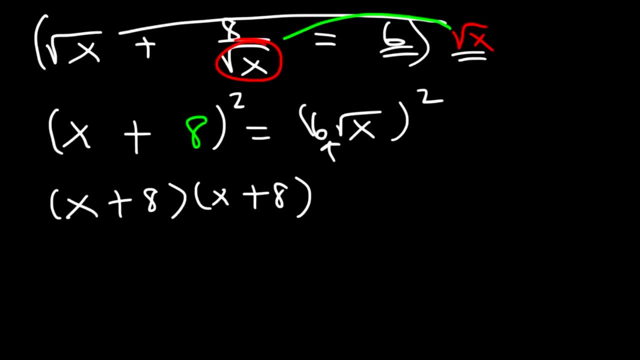 On the right side. we don't have to. We don't have a plus or minus sign that separates the 6 and the square root of X, Because they're multiplied. we can square the 6,, which is 36.. And the square root of X is simply X, so we get 36X. 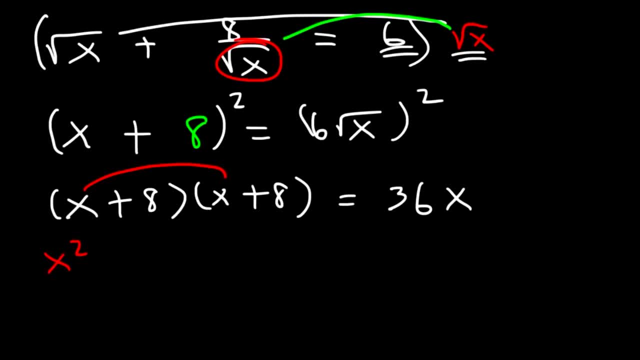 But now let's FOIL: X times X is X squared, X times 8 is 8X, and this is also 8X. And then 8 times 8 is 64.. So, combining like terms, we have X squared plus 16X plus 64.. 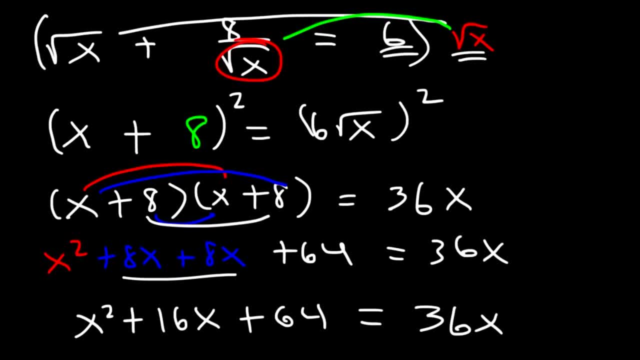 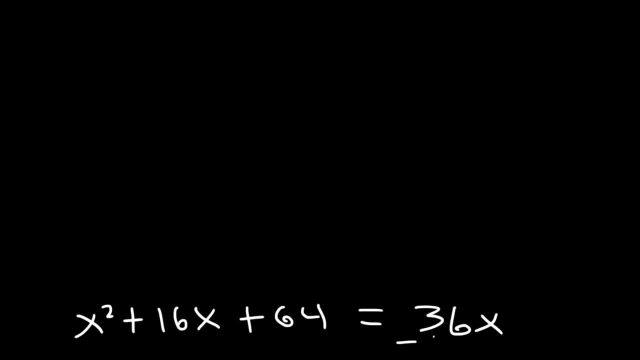 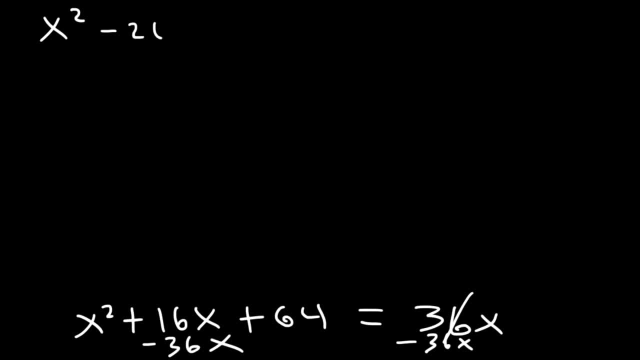 16 minus 36 is negative 20.. So here we have a trinomial with a leading coefficient of 1.. Now, in order to factor this trinomial, we need to find two numbers that multiply to 64, but add to negative 20.. 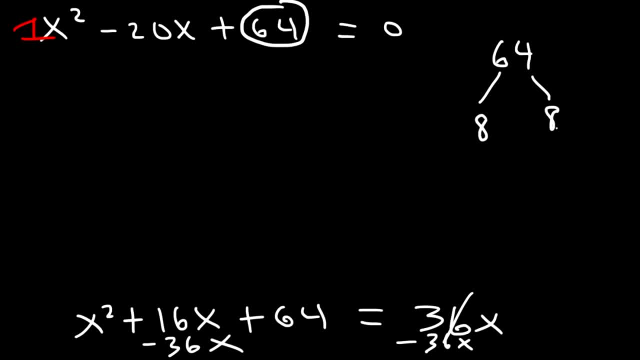 So what are some numbers that multiply to 64?? We have 8 and 8,, 4 and 16.. Notice that 4 plus 16 adds up to 20.. Negative 4 and negative 64.. Negative 4 and negative 16 adds up to negative 20, but still multiplies to positive 64.